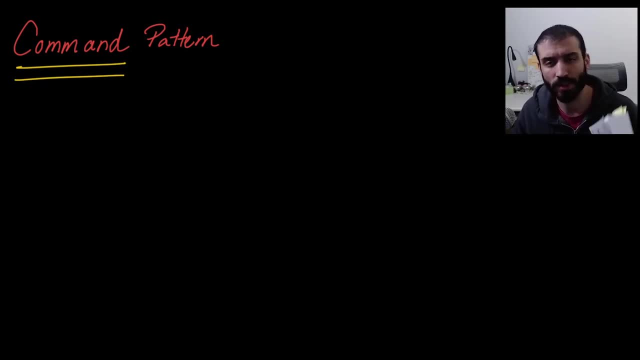 if you haven't checked that out, go ahead and check that out. i find it's a. it's a good, easy read to understand. some of these design patterns gives you some great examples and things like that, so i'd highly recommend it. i'll put a link in the description section below and some of the 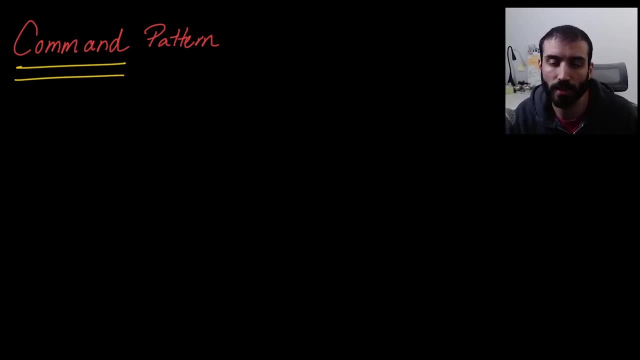 examples that i'm going to use in this video are kind of based on some of the examples in this book, so you can kind of get the idea and follow along if you are reading it as well. so, like i said, in this video we're going to talk about the command pattern and i'm going to first define it. 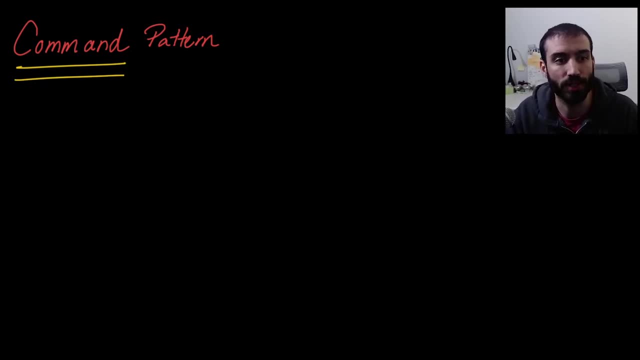 for you it's. it's obviously very important to understand what the definition is. and then we're going to run through an example and then i'm going to show you some of the code in my ide, just kind of demonstrating the example using real classes for a real problem, just so you get an idea. 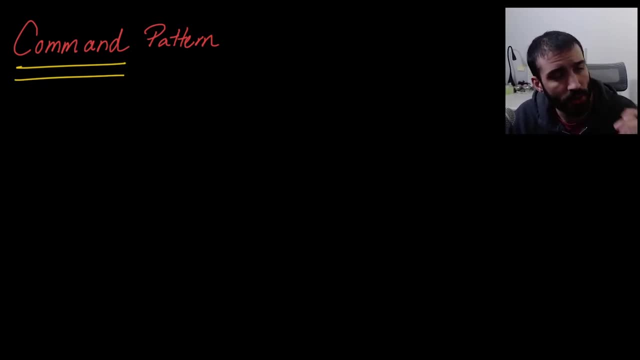 of how it works. so, unfortunately, i found the definition from this book wasn't very good. it was a little bit too basic, so i pulled one off of wikipedia that i thought was a little bit better. uh, so i'm just going to read it out to you and put it on the screen at the same time. so, in object. 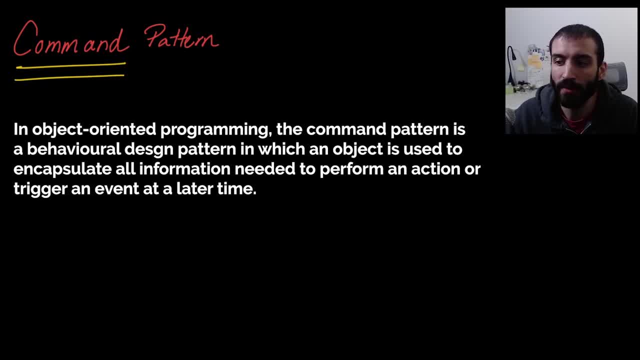 oriented programming. the command pattern is a behavioral design pattern in which an object is used to encapsulate all information needed to perform an action or trigger an event at a later time. this information includes the method name, the object that owns the method and values for the method parameters. um, so that was a little bit of a mouthful, but, and the way that i like to think of. 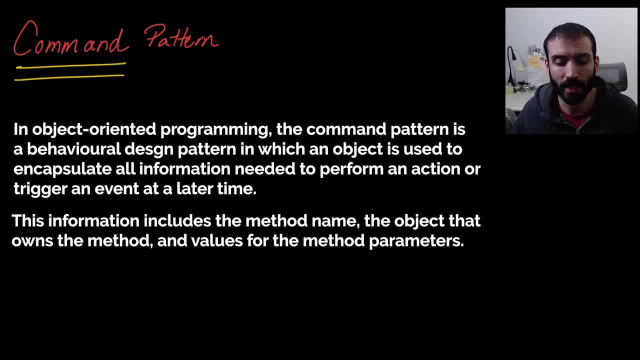 the command pattern is a little bit different than this definition, but i like to think of it in the sense that you can wrap functionality or wrap behavior in a class and in the method and then you can kind of pop that into a slot and that slot is interchangeable with other methods and as long 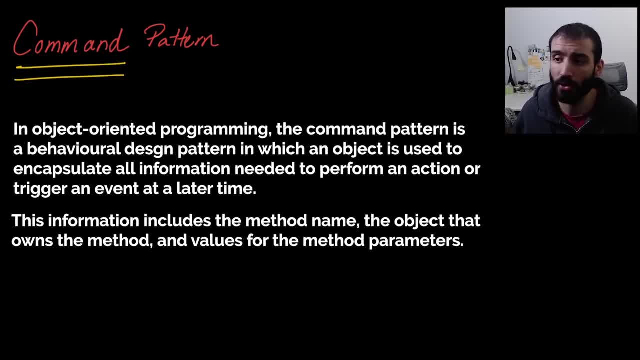 as they're interoperable and adhering to the method, you're going to be able to do a lot of samples in a particular way and they're all able to be routed to the same pattern and they can fit inside that slot. so it's all right. if that doesn't make sense, i want to run through an example with 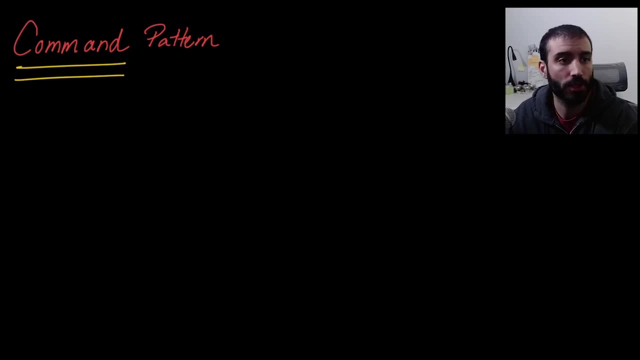 you now, and it's going to be based on a popular home item. so let me just grab the image here and for the example we're going to be using a item that you may be familiar with. this is a amazon alexa. it's a speaker device that a lot of people are using these days and you can kind of 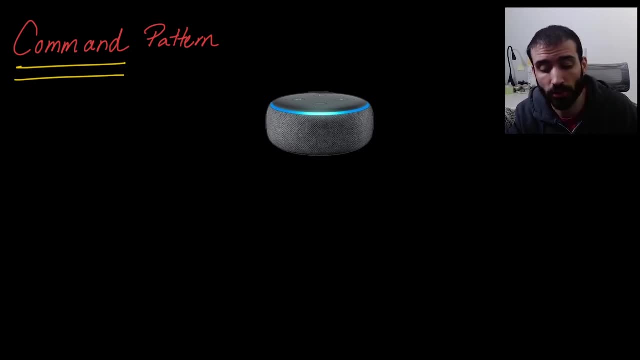 ask it to do things like play music. you can. if you have a really smart house. you can ask it to get to turn the lights on, change the temperature of those lights, And it can do a whole bunch of other things too, like kind of connect to your fireplace. There's a whole bunch of different. 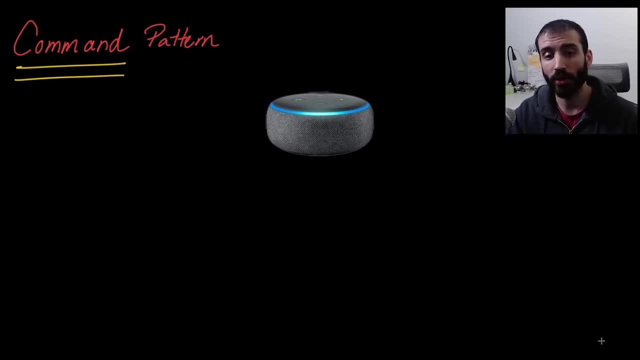 options here. So if you didn't already know, with an Alexa device you can kind of encapsulate a bunch of those different behaviors in one command. So for instance I can say to my Alexa: turn on the music right. And I can encode that to say: oh, a very particular radio station, a very particular. 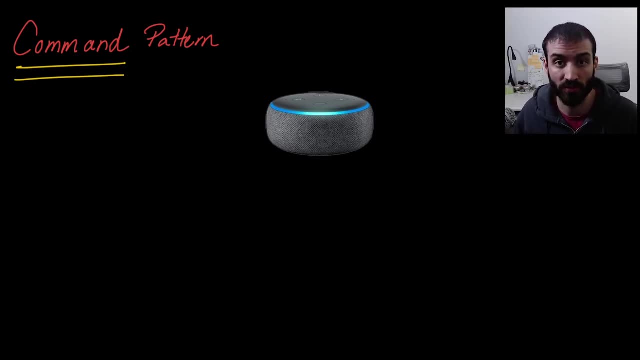 volume setting and a whole bunch of other characteristics of that. I can also combine that with other things. So maybe when I say, turn on the music, I want to turn on all my lights and set the color to red, things like that. And the way that you can imagine this is you kind of have. 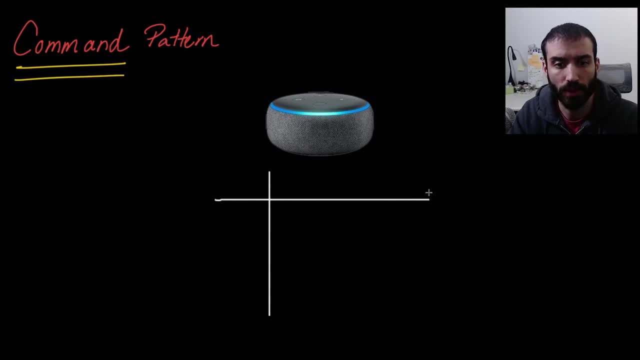 a matrix of possibilities here, of different things that you can do, So let me just draw out this grid here with a couple different commands. Okay, that's looking good, And let me give you some oops. Okay, let me go get some vertical lines. 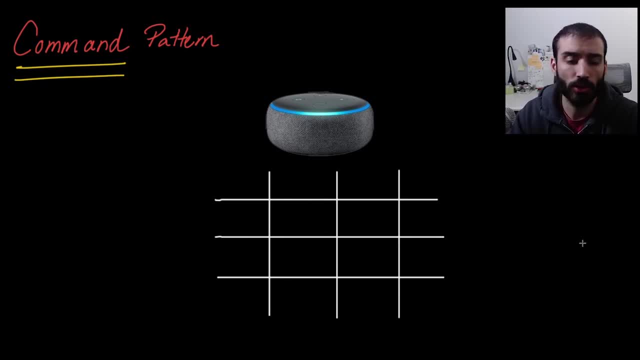 Okay, that's looking about right. So you have this. I'm going to introduce this idea of like slots. right, There's these different slots that you can put things in So you could put like a music command here you can put: you know, turn all the lights off or turn everything off command. 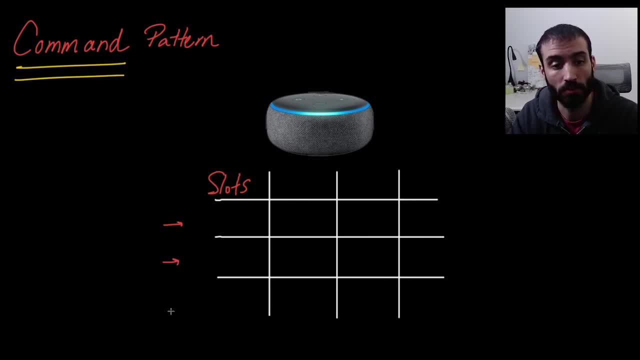 here- There's a whole bunch of different options here- and combine different options and make Alexa basically do whatever you want right Now when you're creating- let me just take this out actually so it doesn't confuse anyone- Now when you're, when you're using Alexa, there's only kind. 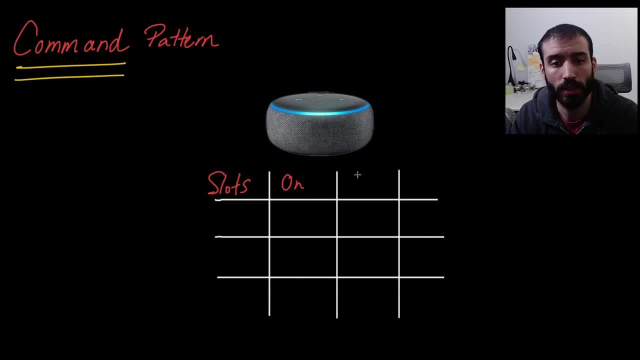 of two states, So you can do whatever you want, right. So you can do whatever you want, right. It's either in an on state or an off state for these you know commands that we're talking about And actually you know what. let me just kind of demonstrate that I want to make be crystal. 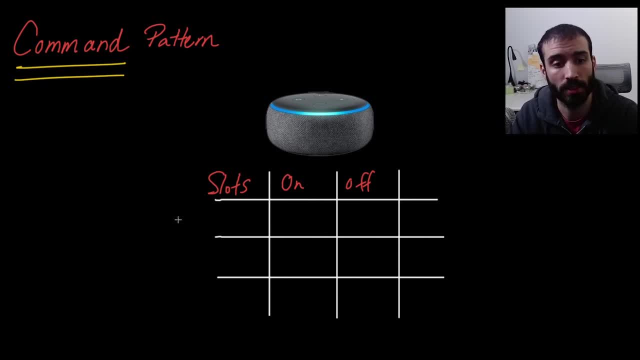 clear about kind of the different things that can encapsulate a single command here. So let's say, like we have a music class or a music command rather, And in order to kind of interact with music, we we can either turn it on or off, we can set volume. 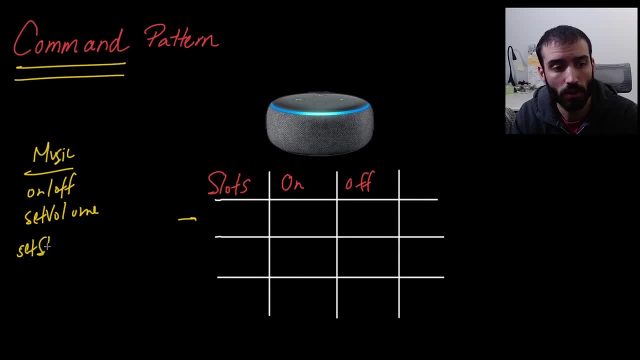 Set volume, we can set station, Maybe we can even like set playlists or something like that. So set playlist. There's a whole bunch of different things that you can do here, But some of these things can be done in combination of one another. So, for instance, you can't set a playlist and set. 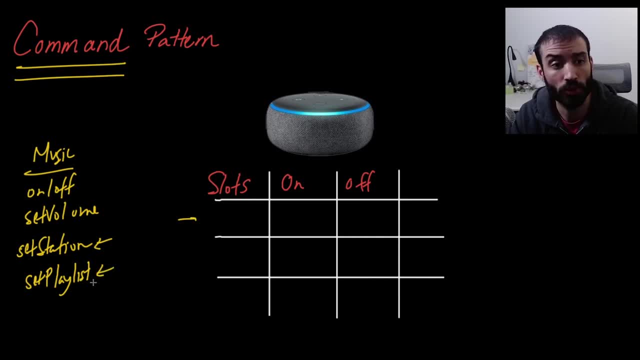 a station at the same time. Those are two separate things, right? So turning your music device on can mean a whole number of things. It can mean, you know, you're obviously setting it to on, maybe, and your station to 99.9, or something like that, right? So when you're defining a slot here, you 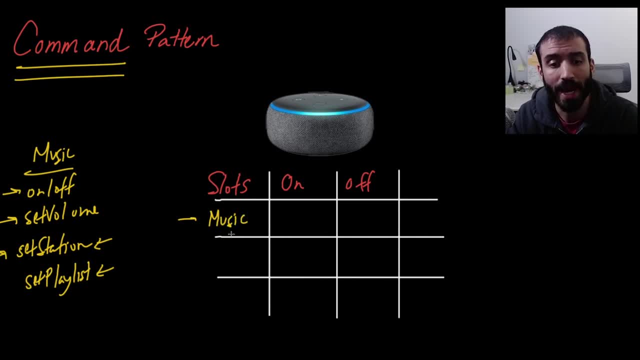 know, your slot might say: play music right, And it may say you can say on here. but what does on actually entail? Well, in this example, it entails turning the device on, setting the volume and setting the station. Now, how do we translate those set of requirements into a binary on or off switch? 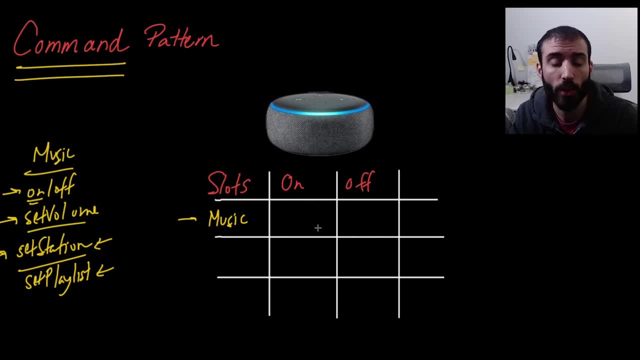 here right? That's really the question that the command pattern helps you solve, And the way that we do that is by creating a class that encapsulates the behavior of the on state and then also encapsulates the behavior of the off state And it's kind of scoped to the particular. 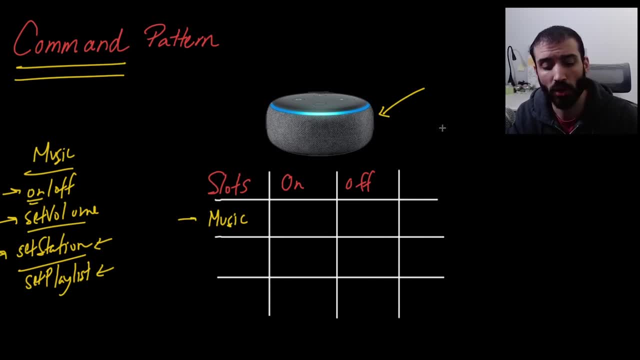 device in question. So that's the general idea of the command pattern. So let's just go through a couple more examples. So we saw the music slot and you know on means you're obviously going to turn it on, So you set volume here, you know, you set volume and then you set station is what we 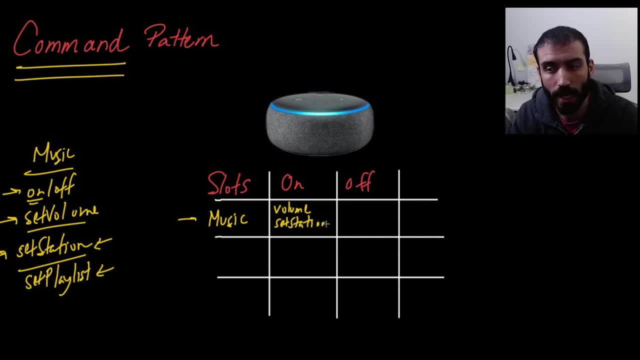 said So, set station or set Frequency or something like that. Okay, so let's get a different color here for the next one. What if we had something like kitchen lights- kitchen lights. Well, this is much more clear, right. 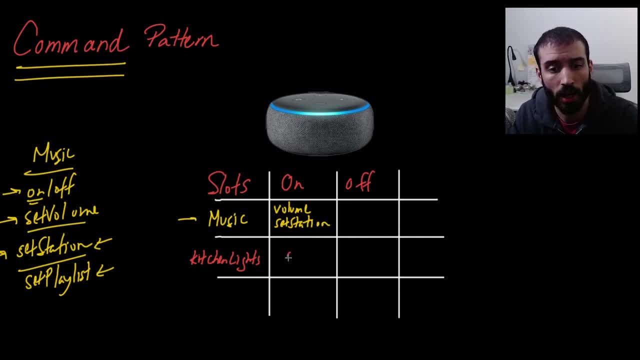 Especially if you have some basic lights. it's probably just you know on or off, So on, just you know goes on and then off, it goes off, Right. So there's no extra functionality here related to kitchen lights. Maybe if you had like different temperature lights where you can set. 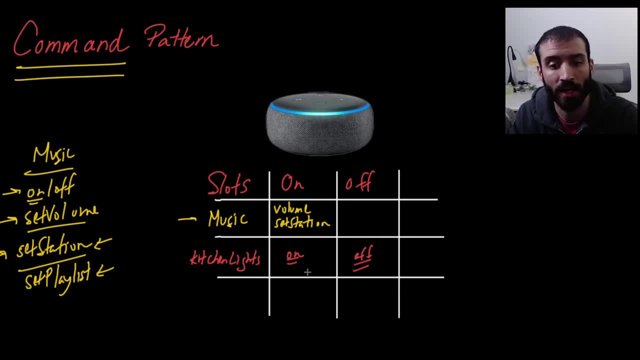 different temperatures and different brightness Levels, then you can kind of combine additional functionality in here. But you can see, in this example I just want to demonstrate that this is like a simple case, that's binary, where it's either just on or off. the same pattern can be used. But the neat thing about the pattern is 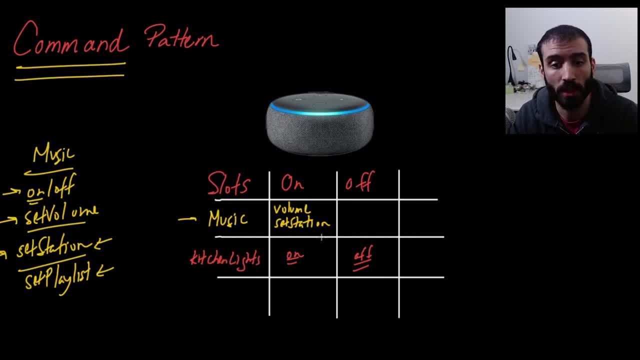 that it lets you kind of encapsulate the on behavior into an object and kind of define whatever that means. Okay, so what happens if we do something else? Like what, if we want to combine these two things? now? So let's say we have like an all setting, like we say: Alexa, turn all the. 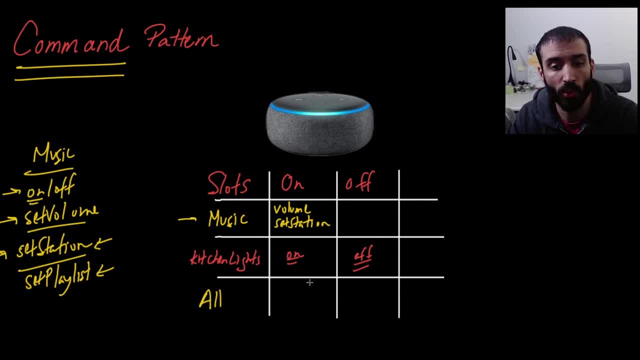 things on right. So then that can mean basically the same thing, But we can combine all this functionality together So we can say: music on right, Music on music volume. I'm just going to write M for music, music volume. We can do music, Maybe in this case. 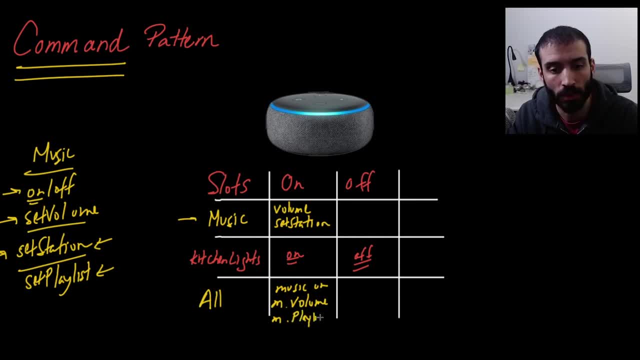 we want to do playlist instead of station playlist, And then we also want to do kitchen lights on right. If we want to combine everything together, kitchen lights on. So you can see, here we're encapsulating all these different behavior into just like an abstraction for on. But you know, 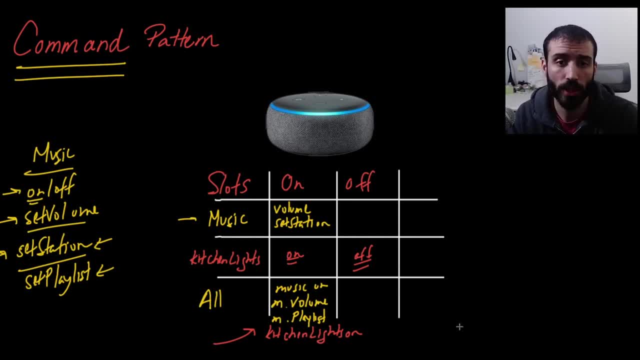 it applies differently to all these different objects. So what I want to do now is take you into my IDE and show you an example of this actually working, So you can see how it works in real life and how some of the interfaces and all that are set up. So I'm going to take you over. 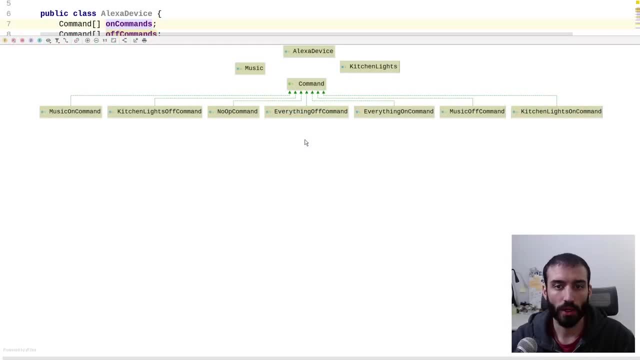 into my IDE now, So I'll see you there. All right, guys. so here we are in my IDE, So I just generated a quick class diagram just to show you kind of what we're working with, so that you can follow along. 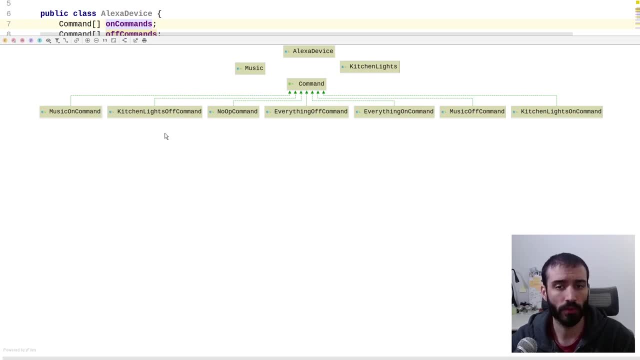 I'll leave this at the bottom so that you can kind of keep track of what's going on as we go through all the code here. But let me just give you the low down here. So, starting from the top, So we have a class that represents the device that we're going to be using to control the different slots In this. 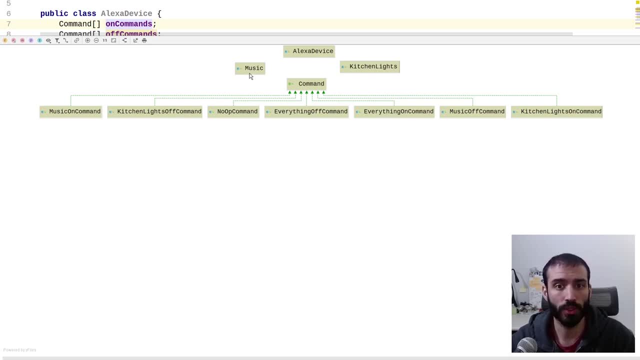 example, we have two different types of hardware. So we have, like, our music playing device here and we have our kitchen lights, And then we have an interface here called command that has one method that must be overridden, And that's an execute method, And we have a whole bunch of different classes here. So let's take a quick look. 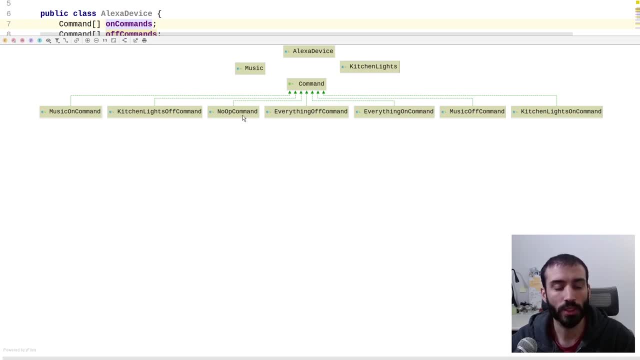 at this. The one that I want to start with is the no op command. That's just a placeholder for our slots so that we don't run into null pointer exceptions. You'll see that in a moment, So let's start from the left now. So music on command. So this is going to be what's activating all. 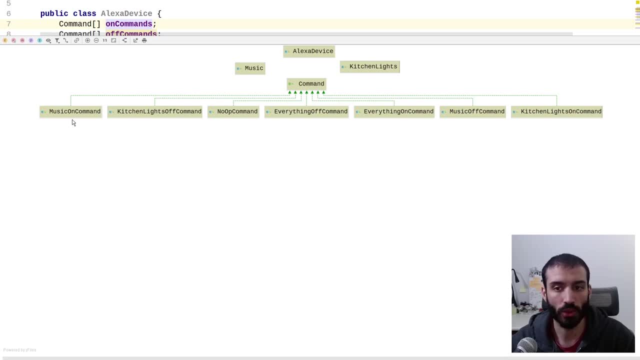 of our music features, things like setting the volume, setting the rate station, things like that. you'll notice that for every on command for a particular type, if we see over here, there's an off command which is supposed to do the inverse of that, And the same holds true for this command. 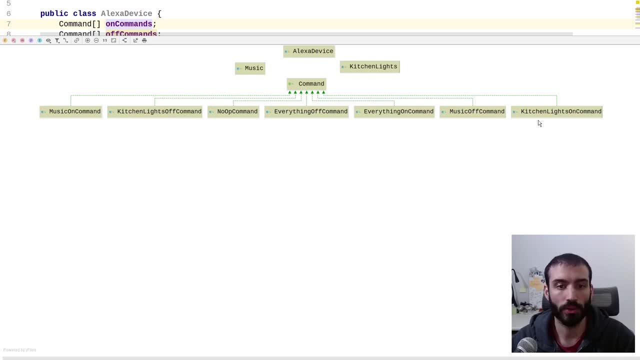 here, the kitchen lights off command, There's also a on command And then finally, like we were discussing in the blackboard section, if you want to turn everything off or everything on all at once, there's the corresponding commands that are going to be used here. So just back to the 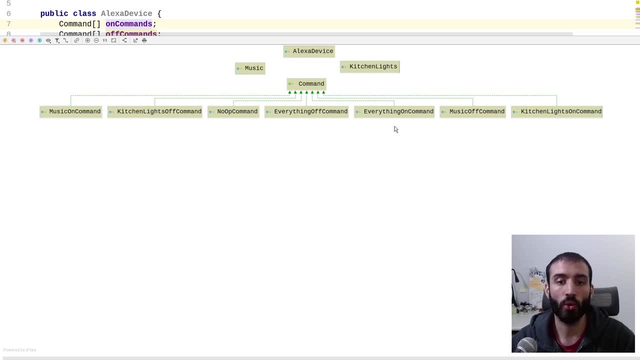 definition. these are the classes that are going to be kind of holding the responsibility and holding the state of activating or deactivating in this case. Now, in this case it's just binary, but it can be multiple things. there can be three different levels of on this or offness And you. 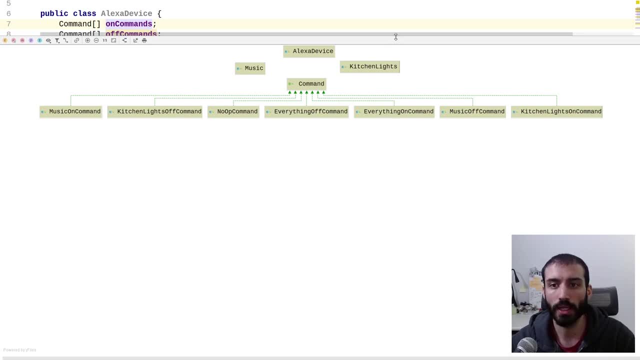 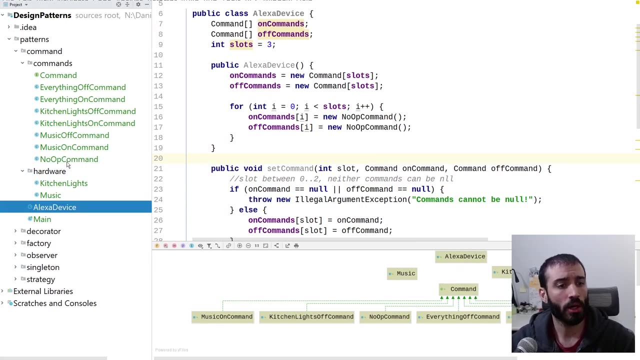 can kind of encode that into your system. So let me just bring this down to the bottom now. So I want to keep that here for the duration of this, just so everyone can follow along. So let's take a look at our classes over here. So what do we got going on? So actually, let's start with our 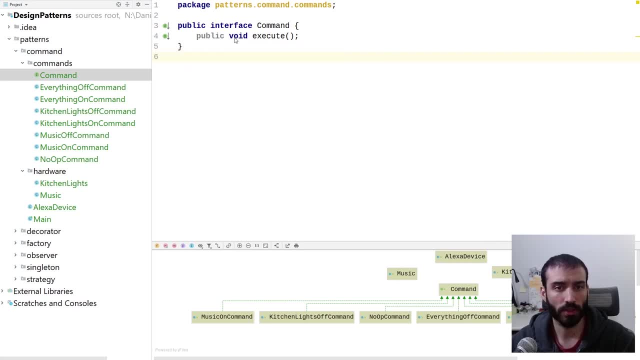 command because it's very simple. So, like I said, we just have a basic interface. all it has is one method, which is execute, And all the other classes that we're seeing here- the off command, the music on off command- all this stuff is all implementing this command interface. So, 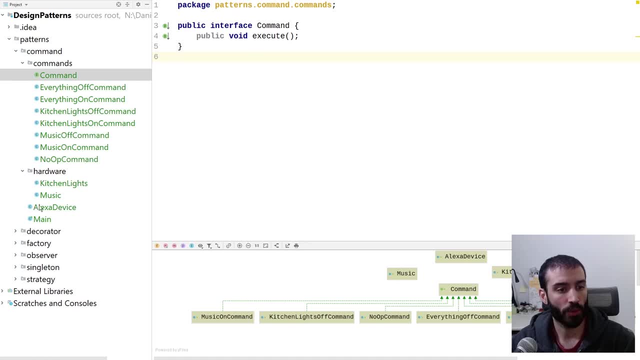 they are all going to have an execute method. Now, before we go into each one, I just want to kind of cover the hardware that we're talking about, because we're talking about kitchen lights on or off, we obviously need to know what the kitchen lights themselves do. Very, very basic I was. 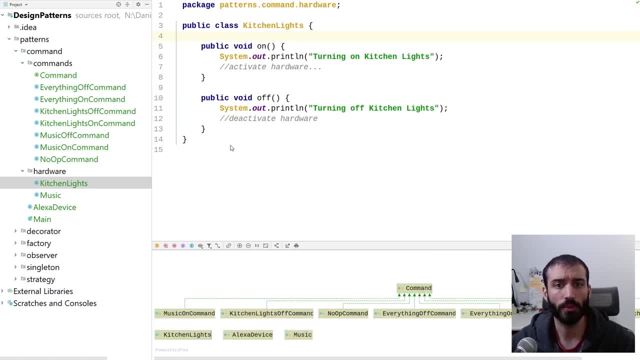 going to add a brightness property here, but I opted to just keep it simple. So you can see. this example is very, very simple. So I'm going to say, if I set it to black, I should be able to see here it will be finished so that we can see. 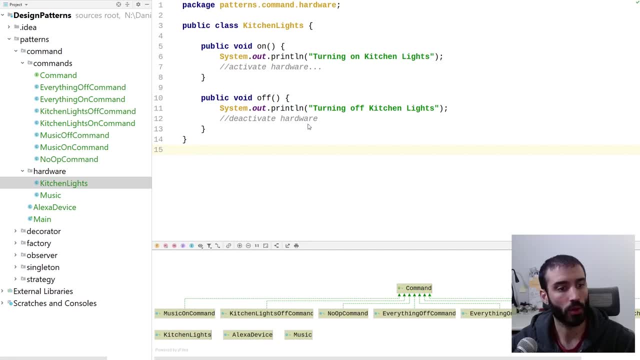 the screen. but again, it's up to you. it's up to you what you want to do here. So I want to show you the controls that we come across in here. So, like I said, I'm going to go to our. 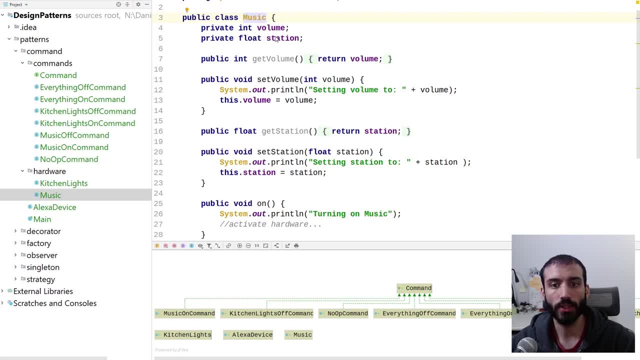 configuration interface And I'm going to type in the name and theID And it's going to show me where it is and then it will take me to my default settings. So there's a lot of information that I need to do here, So let's go ahead and get this done. So I'm going to go back to my 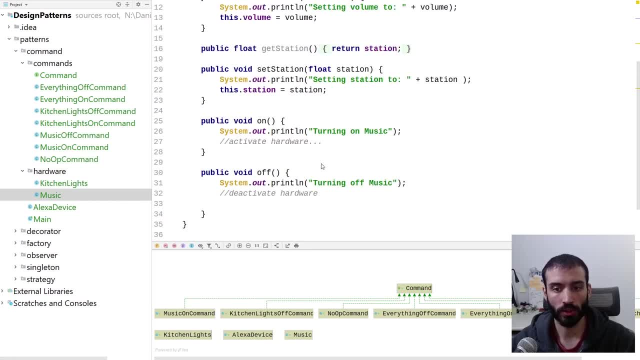 default settings, And then I'm going to go back to the other contacts And then I'm going to go that binary on or off, And we're also printing out what's going on again. So let's go through the different types of commands now, starting with the most simple. So the most simple was: 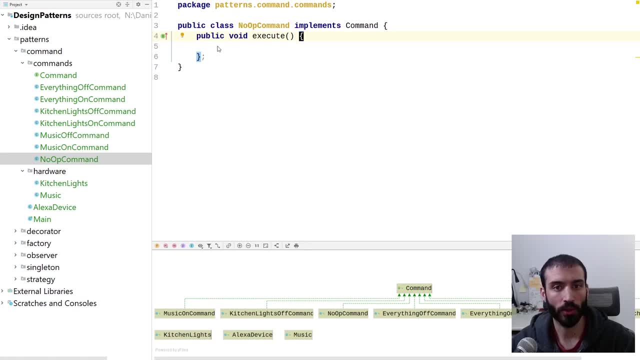 just a no op command. Like I said, it's just a guard against null pointer exceptions. We'll see that in a moment. The second, most simple, is the kitchen lights, And we can see here. there we go. We have a reference to an instance Well before that. actually note that we're implementing that. 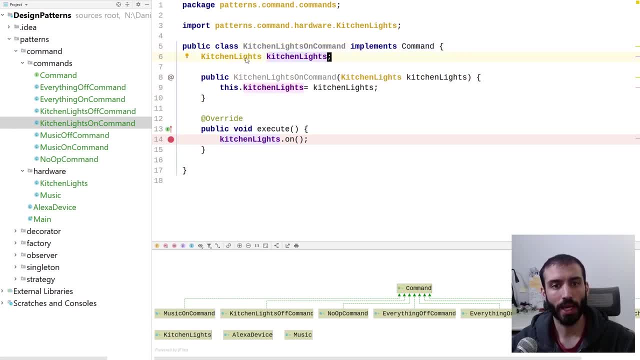 command- So I wasn't lying to you in the beginning- And note that we have a kitchen lights instance that's available to us And that's passed in through the constructor. So when this command is instantiated, it's always with regards to a particular instance of kitchen lights. Now this 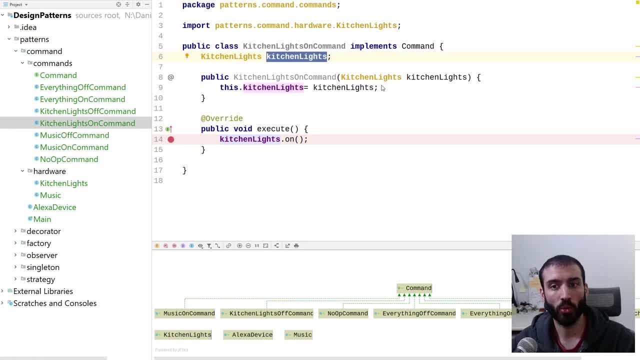 usually you only have a home with one kitchen, But you know, if you have a home with multiple rooms- and maybe your command was room lights on- you may want to know which room you're talking about. So that's why it's good to have the instance in question attached to the. 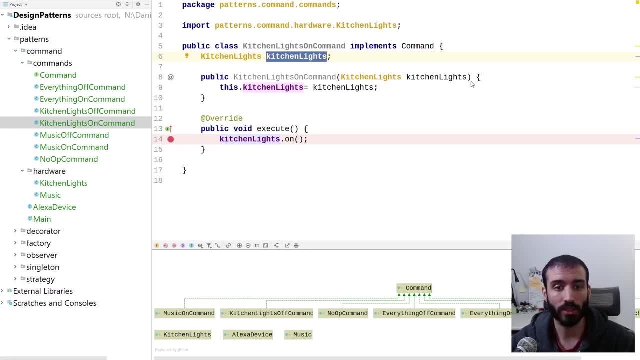 command object so that it can perform the corresponding actions on it. And you can see here for the execute method that we're overriding, it's just very basic, predictable thing. This is a kitchen light on command, So we're going to be turning it on And conversely in the kitchen. 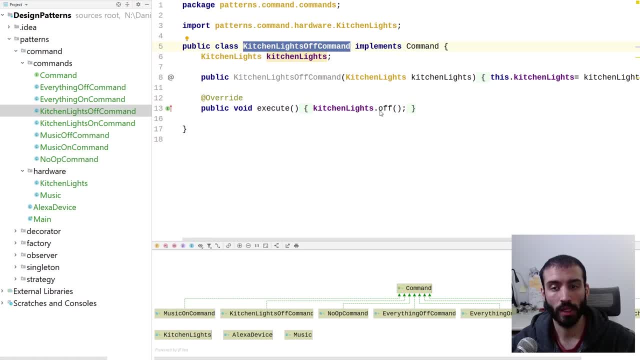 lights off commands. kitchen lights off command. we're going to be turning kitchen lights off. Super simple, easy to follow. Let's take a look at music here. So actually music on rather is a little bit more of a. So now what happens if we want to combine these different things into a particular slot? for instance, I want to tell Alexa, Alexa, turn everything on in my house, right. So that's where the everything on command comes in. So you can see here in this, 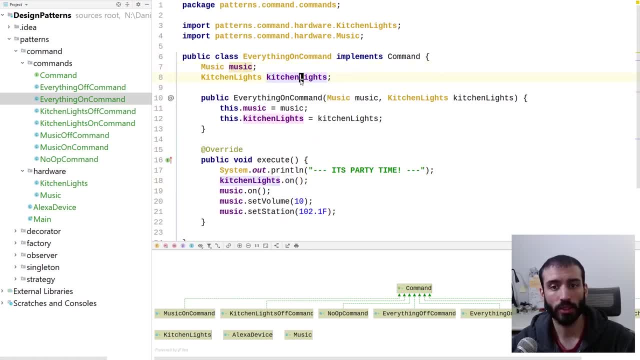 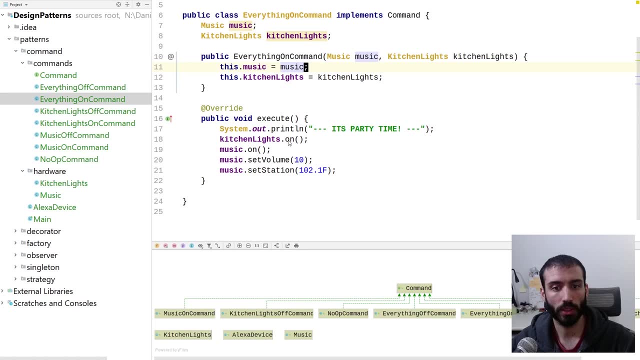 command. we're taking in references to both the music and the kitchen lights, passing that into the constructor, as we see here, And then when we execute- you know I'm being cute here, it's party time- we're using the methods available to us for both of the objects that are 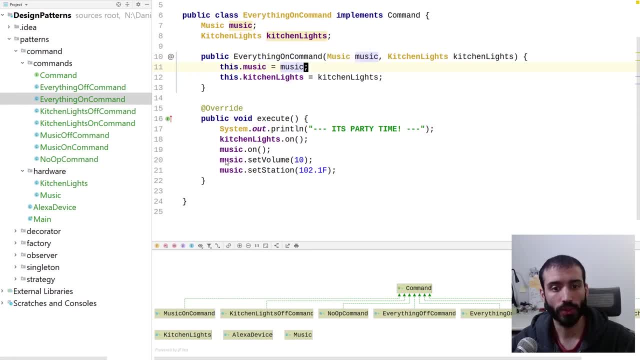 being passed in. So we're turning the kitchen lights on, we're turning our music on, we're setting the volume to 10.. And we're setting the station to my favorite radio station. So you can see here that, regardless of what we're going to get into the slots when we 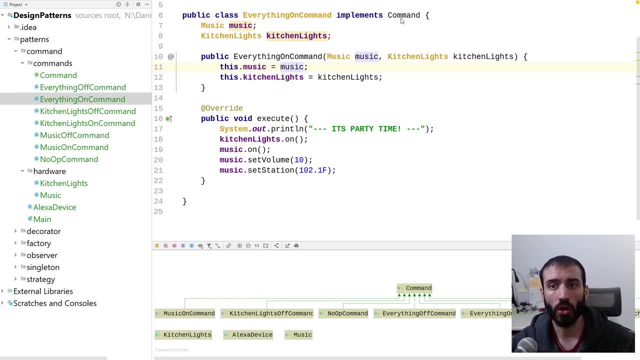 look at the Alexa device. but what should be clear is that since we're all conforming to this, the single interface, these different commands are interoperable, So you can kind of put them in different slots in different states at different times and just remove one pop in. 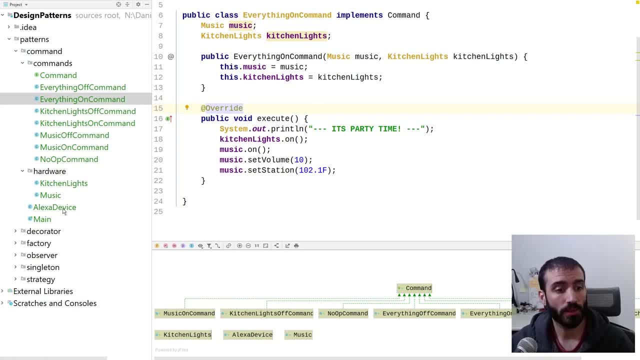 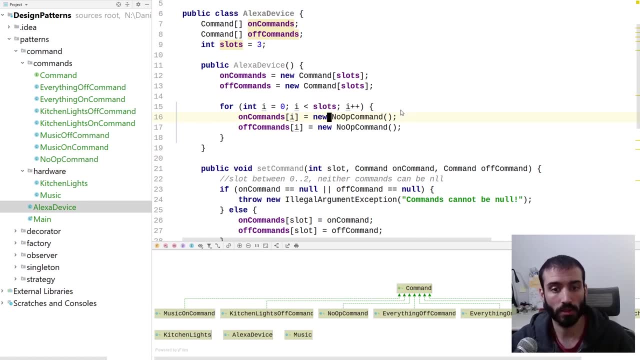 another, and everything just kind of works pretty seamlessly. So in terms of the Alexa device. now, this is where kind of some of the magic happens, in terms of the slots, so to speak. So we can see here that we're holding an array of on commands and off commands. 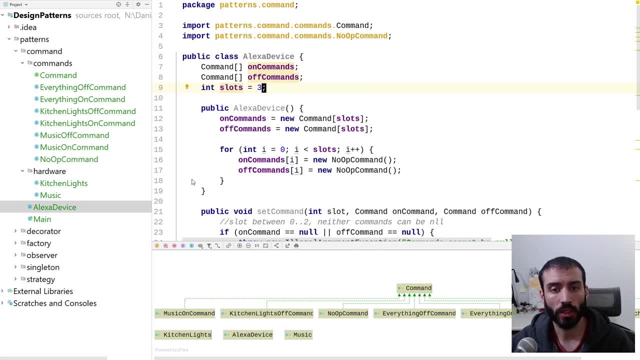 we're setting our slots to three in our constructor here. what are we doing? so? we're creating a array with you know size, slots, length for both on and off, And then we're looping through each and we're just setting them initially to a no op command. This helps protect us from no pointer. 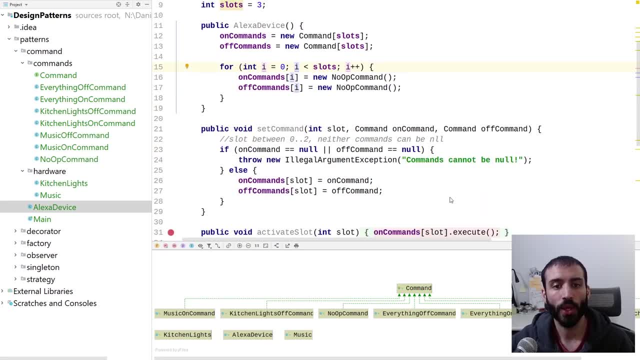 exceptions. Like I said, we're going to see that down below in a second here. Our next method is going to be called during the main method. that actually kind of sets up the Alexa device, And so what we're saying is okay for slots. 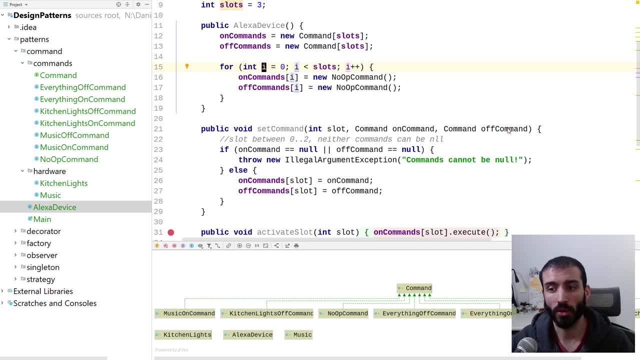 whatever, we want the on command to be this and the off command to be this, So you can start seeing how this is interoperable, right? So you can say: for slot one, you want kitchen lights on, kitchen lights off. For slot two, you want you know something else here and something else there. 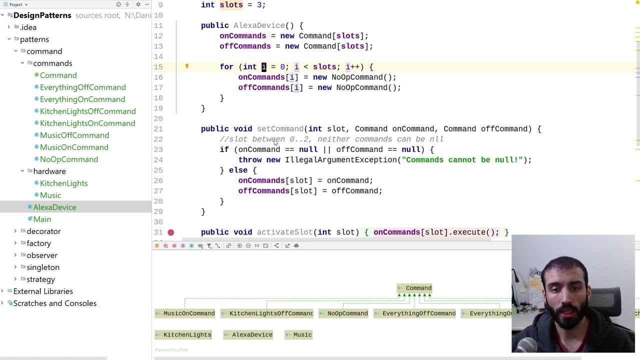 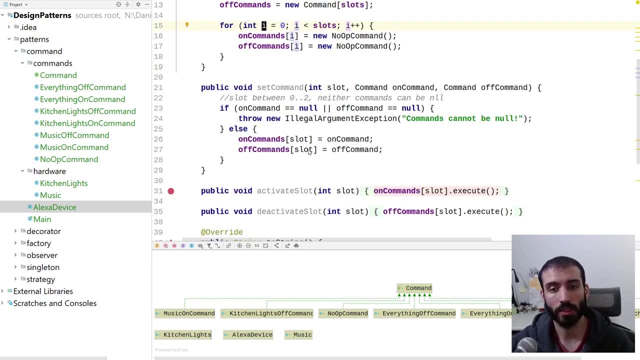 And taking a look a little bit further. we're just checking to make sure on command or off command aren't null, or else that'll cause a problem. So we just throw an exception And then we're just setting the corresponding slot, the corresponding slots on or off command. 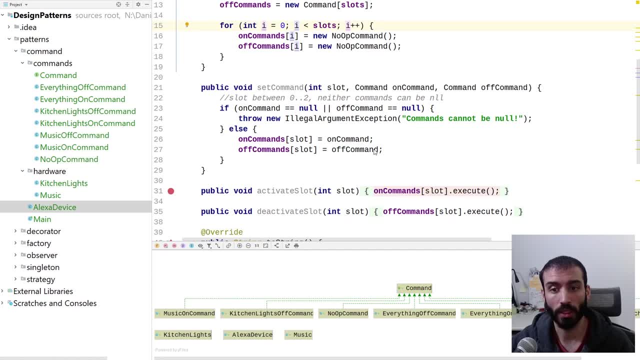 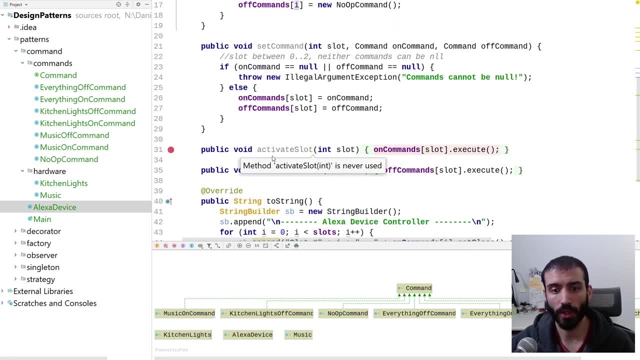 to the corresponding argument that was passed in the on being the on and the off being the off. So far, so good. Next one: we're looking at the activation here, So we have an activate slot or a deactivate slot, rather, And we're just calling the execute method on the instance of the command. 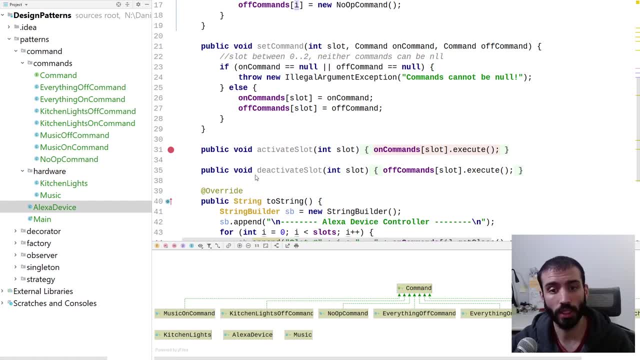 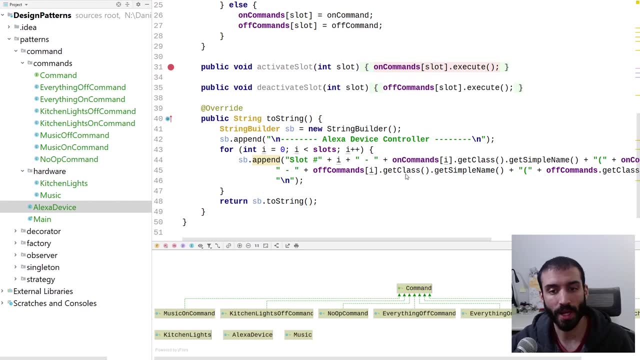 that is in that slot And the same is true for the deactivate slot method And then down here for the to string. I'm just doing something in a nice formatted print way So you can see for each slot what are the commands in this slot for the on and what are the commands in the slot. 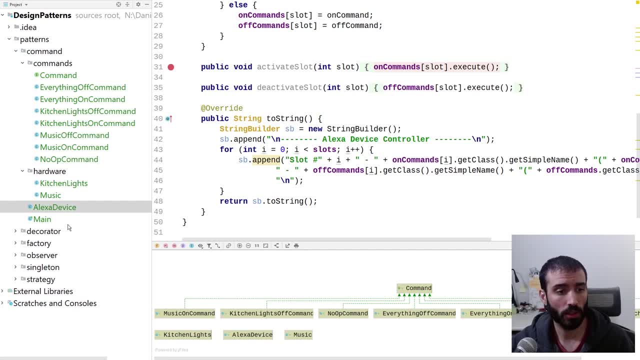 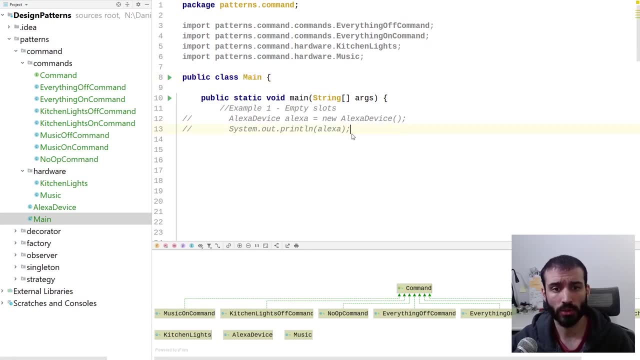 for the off. So that's essentially what's going on here. So let's take a look now at our actual main class and go through a couple examples of how this all fits together. So in our first example- super simple, and I just want to kind of demonstrate to you what's going on- 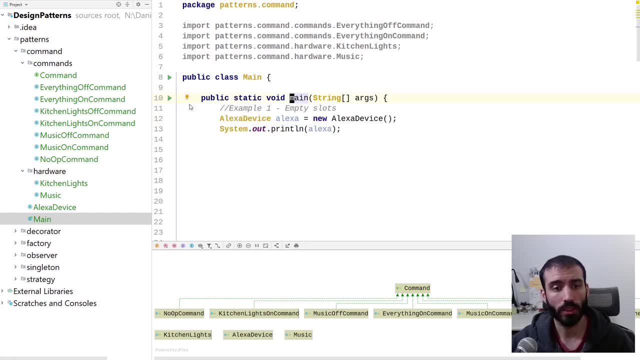 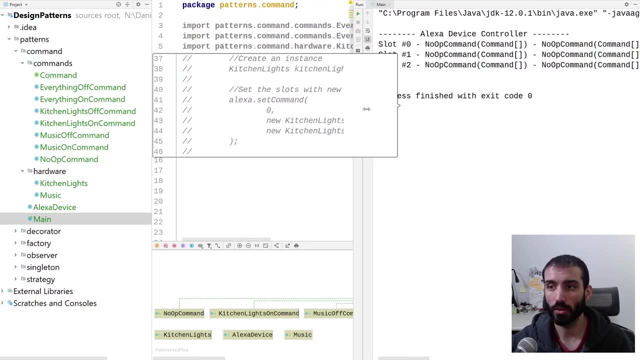 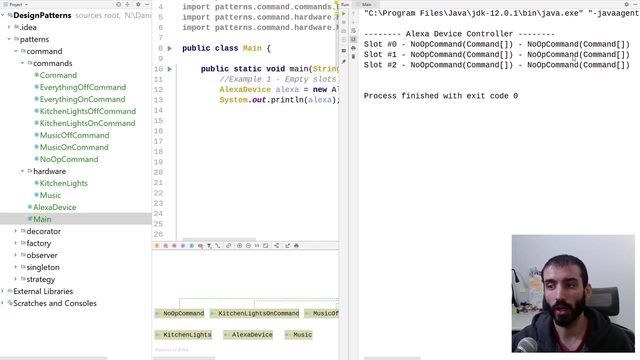 So let's just print this out. So we just have a new Alexa device and we're printing out the Alexa, So this is going to be calling that to string method. Let's run this guy and see what happens. So we have slot zero, no op command, everywhere right, So everything's looking good. We don't. 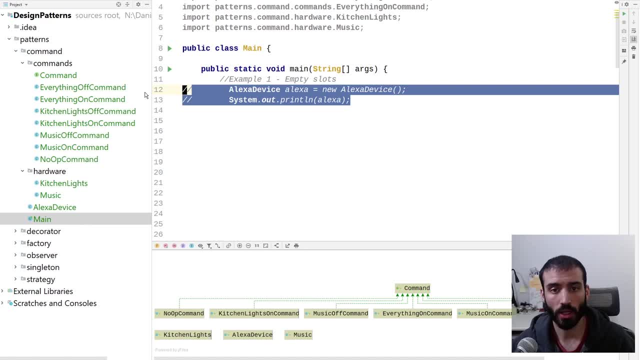 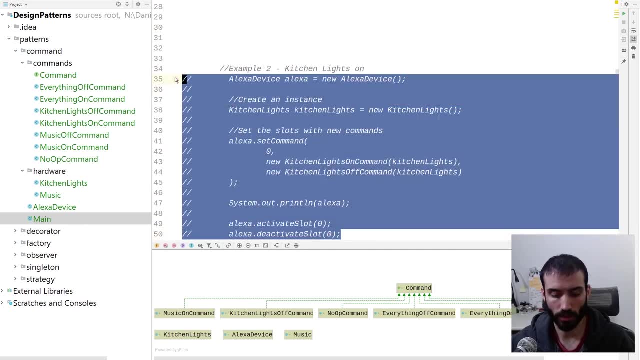 need to worry about null pointer exceptions. That's great. Let's just comment that out now and move down to some more interesting examples. So what do we got going over here? Comment this stuff out so we can see what's happening. And I need some imports. Fabulous Import class, Yeah. 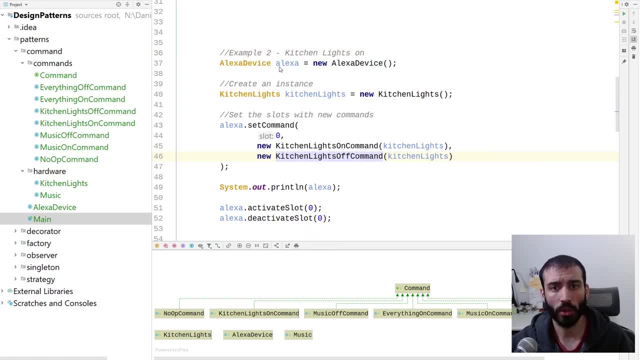 that looks good. Okay, so what are we doing here? So we're going to do the same thing. We're creating a Alexa device, We are creating an instance of the kitchen lights because, remember, we have to take that in as arguments to our on or 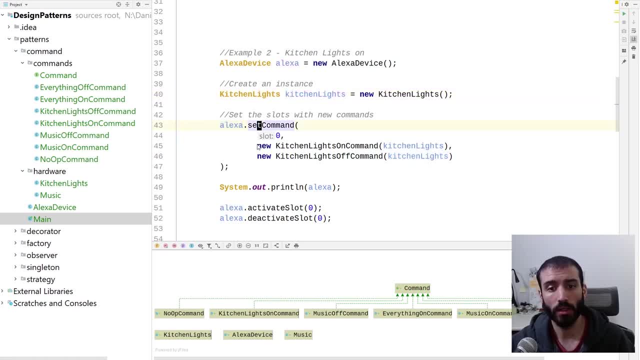 off commands And then we're calling our Alexa devices command center And we want to say, for slot zero, we want to do the kitchen lights on command for this instance of kitchen lights And then the same thing for the off state, again passing in the same instance. Then we're just 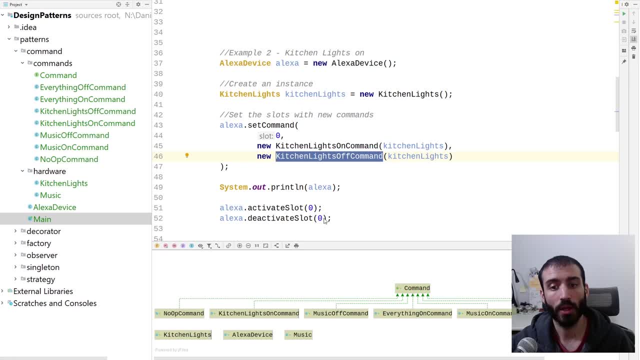 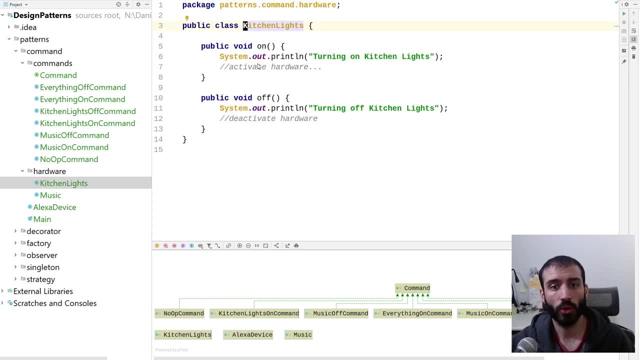 going to print all this out And then we're going to call the activate and the deactivate method of this Alexa device And, if you recall, over here on the kitchen lights, when it goes on or off, we should see turning on kitchen lights, turning off kitchen lights. So that's the expectation. 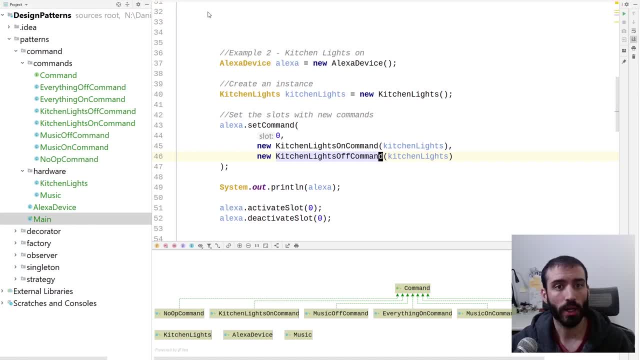 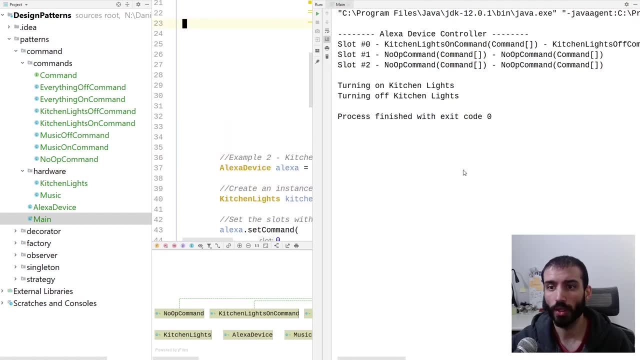 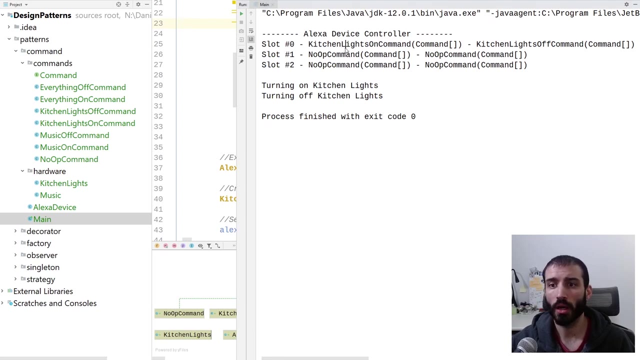 Going back to main. rather, let's see if this all worked correctly run and then I'll pull this out. So what do we got going on here? A little bit more. So we see at the top for device controller for kitchen lights on command is now present. That's great. And kitchen light off command is now. 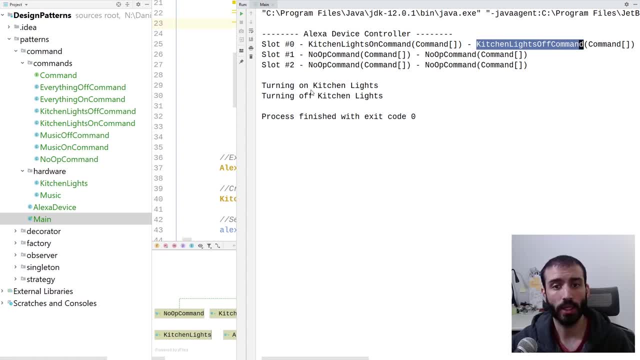 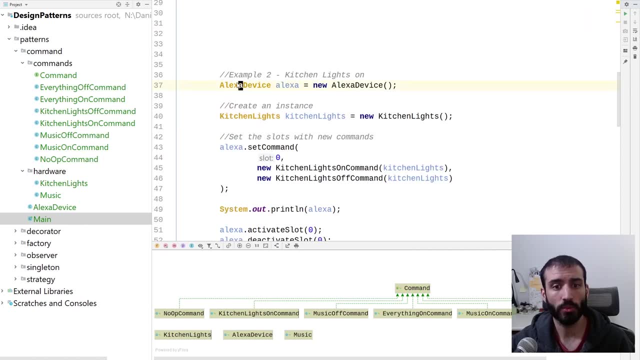 present. That's great. We see, when we ran the activate command, we turn them on, and then we ran the deactivate command, we turn them off. So far, so good. Everything is pretty predictable. Let's move on to the final, more interesting example, which combines: 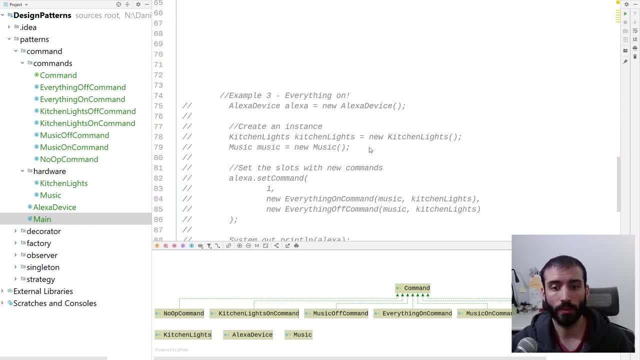 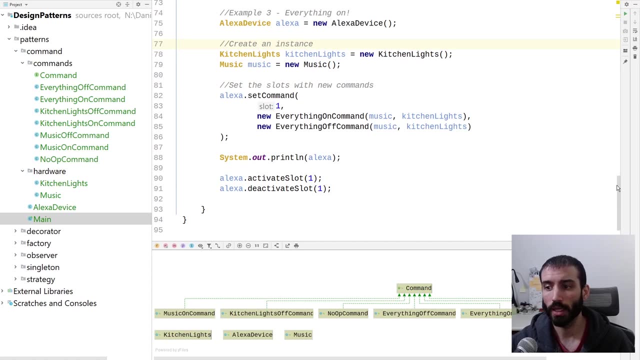 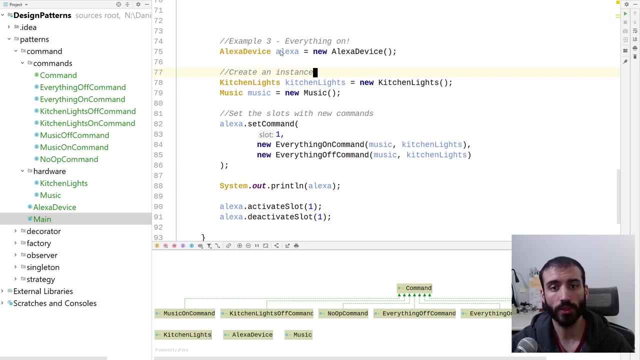 multiple different pieces of hardware together. So let's scroll down. Here we go. Let me scroll up here and uncomment And center this so everyone can see. Okay, perfect. So this is kind of like the party mode, where you want to turn everything on all at once. So again, we're creating a reference. 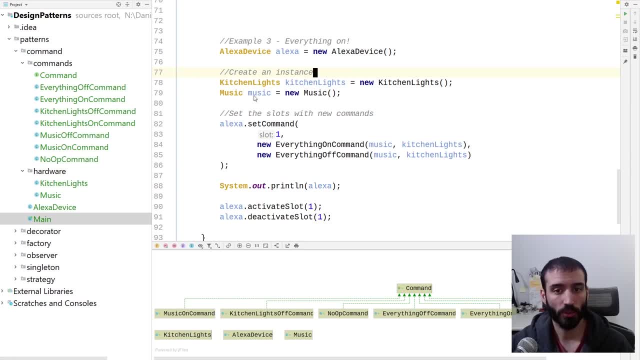 to our Alexa device. we're creating an instance of our kitchen lights and our music And then we're setting the command in slot one this time, And we want to use the everything on command And that's gonna basically call the. the music set volume to. I believe I put five or 10, I can't. 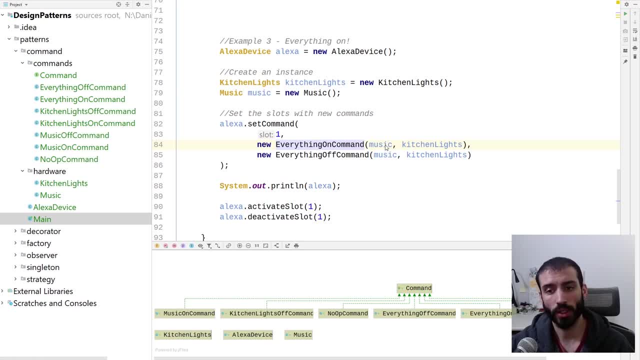 remember, set the station to whatever it was being set to, so on and so forth, And then we're going to turn everything on And then in the everything off command we're doing the opposite of that. we're going to print it out and then activate and deactivate. When we activate, we should see 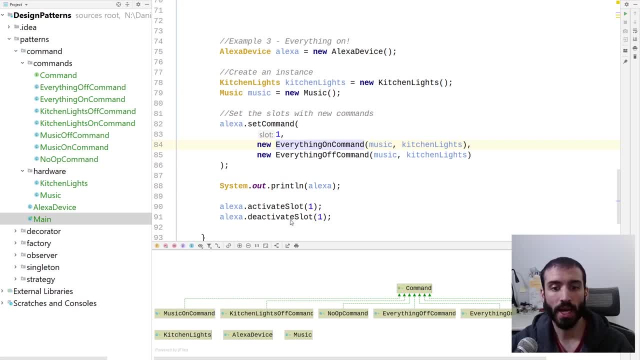 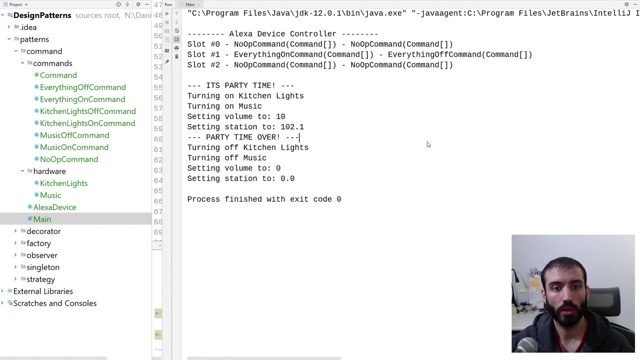 its party time and everything turning on. And when we deactivate, we should see party time is over and everything turning off. So let's just give this a another run now and just verify what happened. Oh, I need to pull this out, don't I? Okay, so what do we have here? 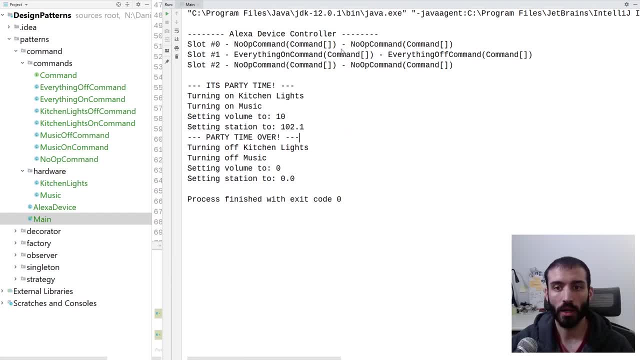 So slot zero is empty great. slot one is everything on command, everything off command, perfect. And then when we activate it, we see it's party time. we're turning on the kitchen lights, we're turning on the music, we're turning the volume to 10, setting the station to my favorite. 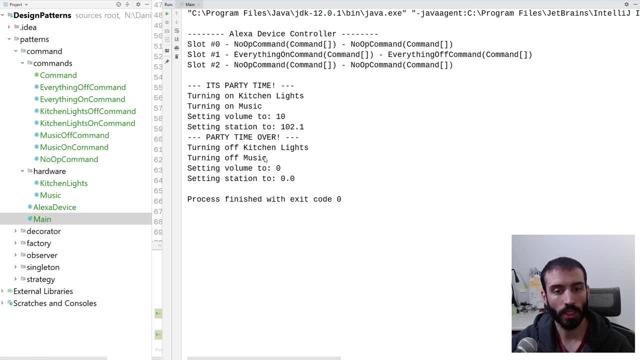 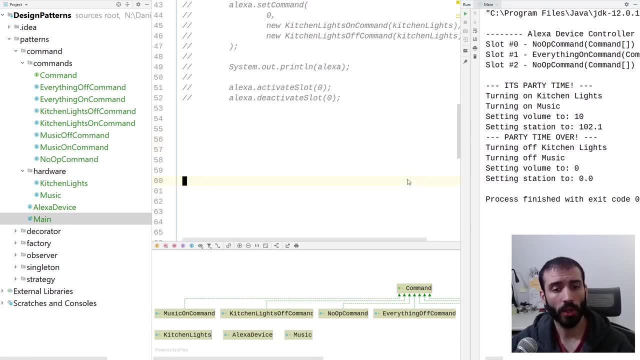 station And then, unfortunately, party times over and we are turning everything off. So we're seeing here that everything was working correctly. I'll make this code available to you below, But hopefully it's clear Again by looking at the diagram here at the bottom.